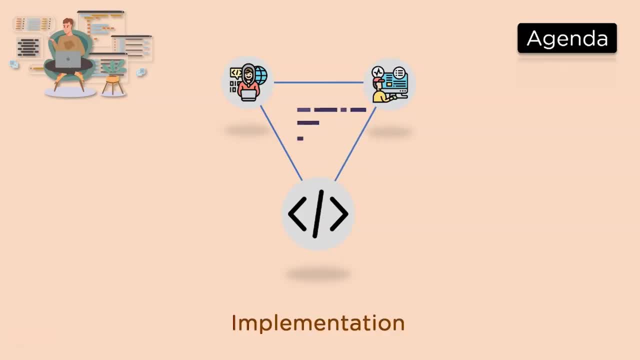 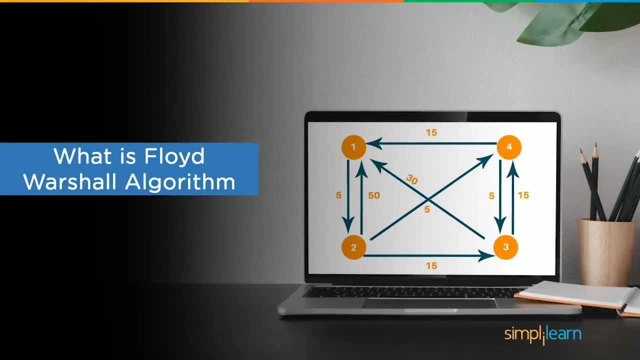 algorithm to solve all pairs shortest path problem in the code editor. But before we begin, make sure you have subscribed to our YouTube channel and clicked on the bell icon below so you never miss an update from Simply Learns YouTube channel. So without any further. 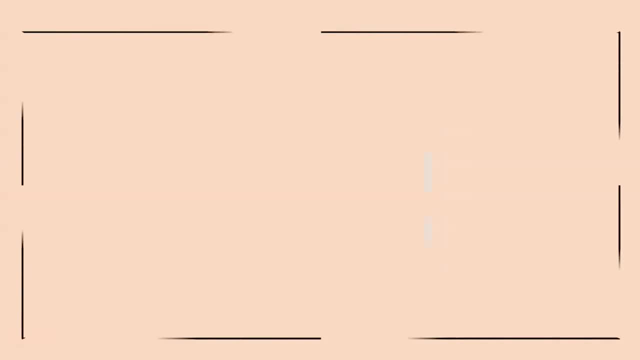 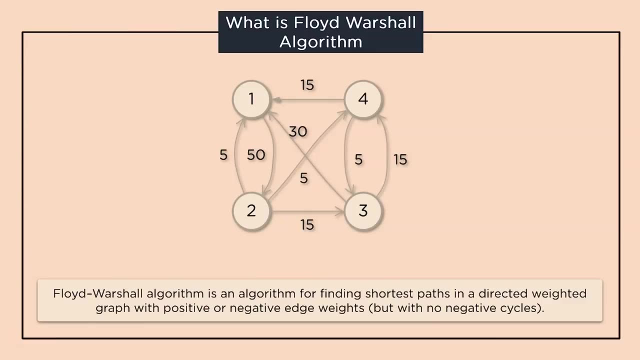 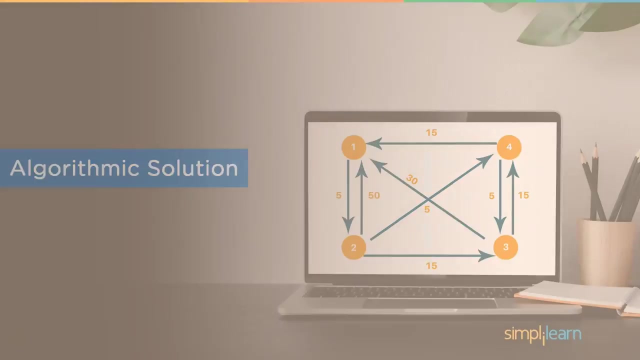 ado. let's get started with the topic. what is Floyd-Warshall algorithm? The Floyd-Warshall algorithm is for solving the all pairs shortest path problem. The problem is to find the shortest distance between the two pairs. Now let's discuss the algorithmic solution to the all pairs shortest path problem First, 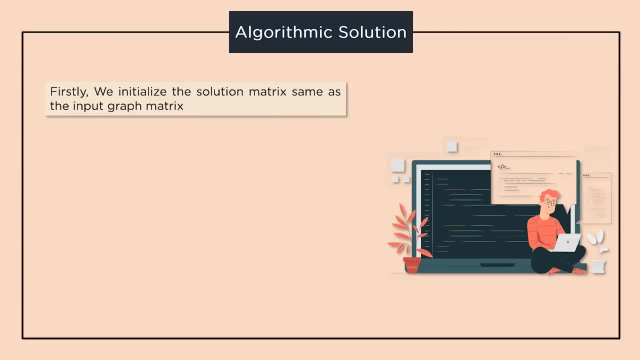 we will initialize the solution matrix the same as the input graph matrix. Then the solution matrix is then updated by treating all vertices as intermediate vertices. Our main goal is to pick all vertices as intermediate vertices. We have now discussed the Floyd-Warshall algorithm and the algorithmic solution to all pairs. 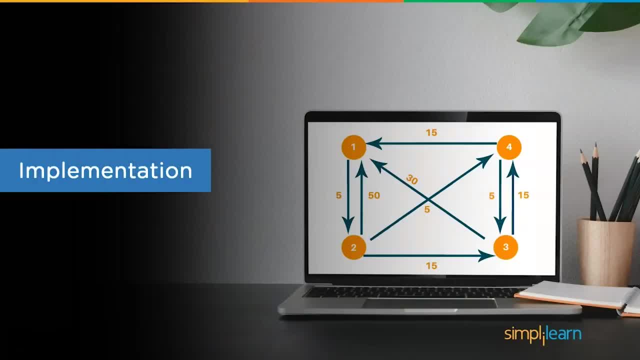 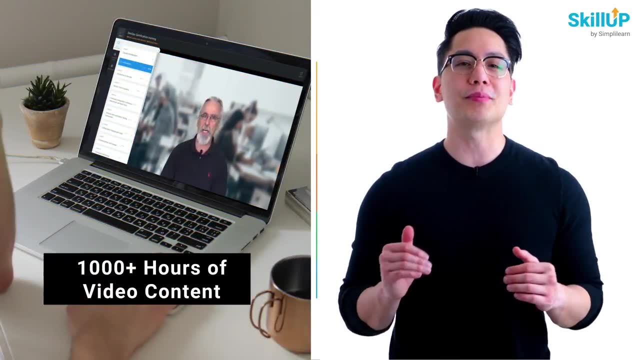 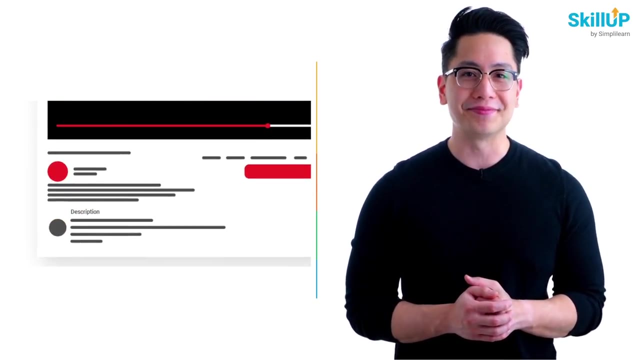 shortest path problem. Now let's implement this solution in the code editor. Choose from over 300 in-demand skills and get access to 1000 plus hours of video content for free. Visit SkillUp by SimplyLearncom. Click on the link in the description to know more. 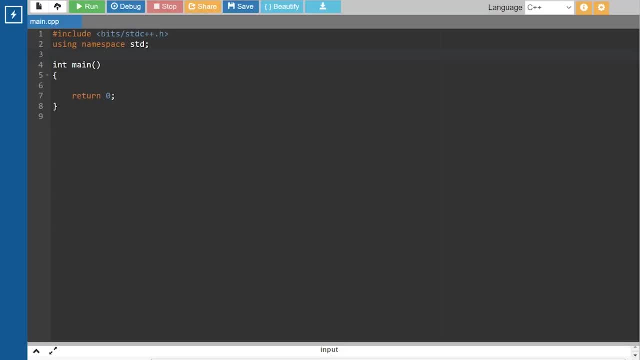 We will start by defining vertices. We will have four vertices. So hashtag: define INF, which will be equal to 9999.. Now let's write a function to print the solution matrix. So void: print solution with argument as int: two-dimensional array test. So the argument: 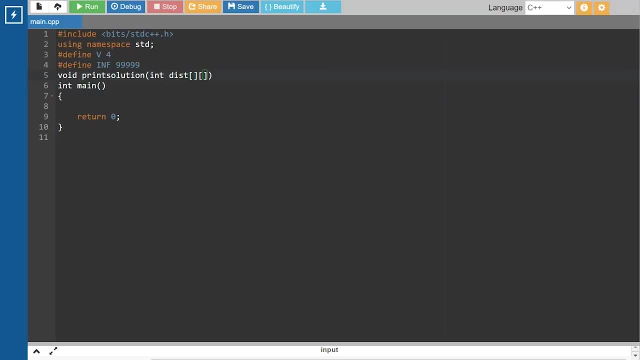 is int two-dimensional array test. So the argument is int two-dimensional array test. So the argument is int two-dimensional array test With its y as v. we will come back to its definition later on. Now we will write a function to solve all pairs shortest path problem using Floyd-Warshall. 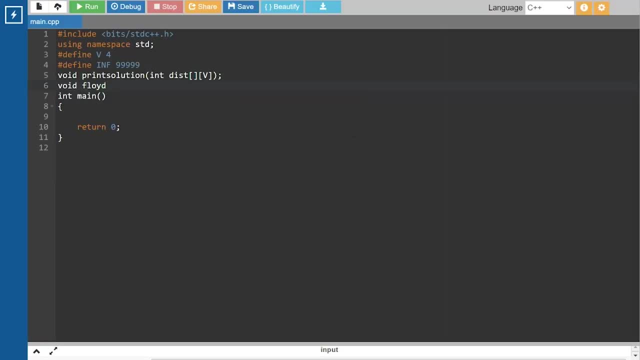 algorithm. So void floyd-warshall int graph. This will also be the 2D array which has y as v. Now we will define dist 2D array. It will be the output matrix that will finally have the shortest distances between every pair of vertices. 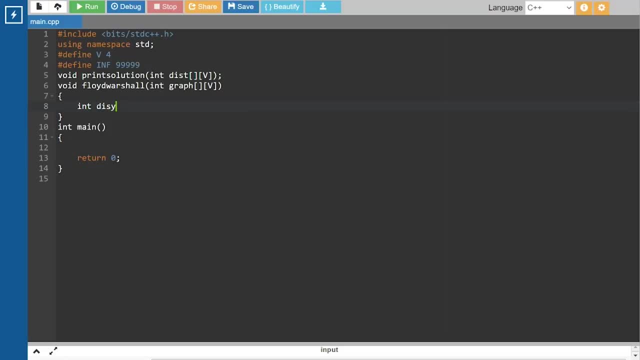 So int test its x and y will be vijk. Now we will initialize the solution matrix same as input graph matrix. Or we can say that the initial value of shortest distances are based on shortest paths, considering no intermediate vertex. So for i is equal to 0,i less than capital Vi plus plus. 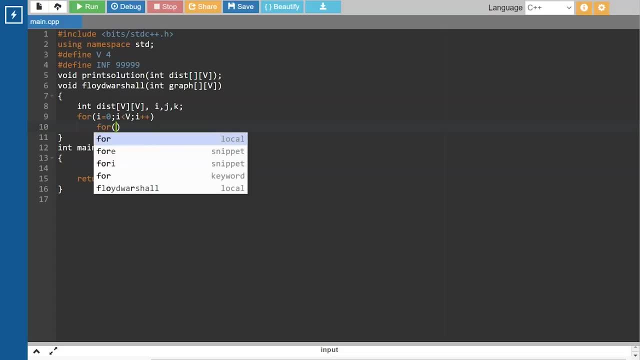 Another nested loop for j is equal to 0,j less than Vj plus plus. So distance at i comma j will be equals to graph at i comma j. Now we will add all vertices one by one to the set of intermediate vertices, So before start of an iteration we will have the shortest distances between all pairs of vertices, such that 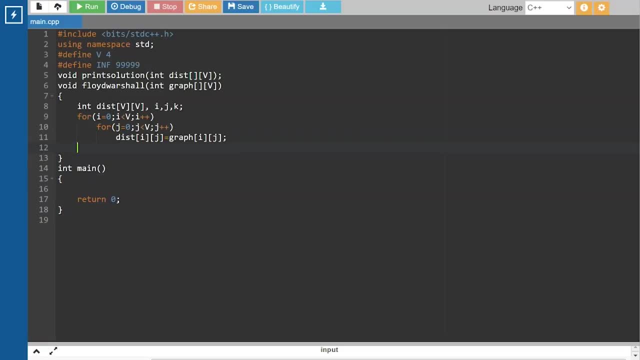 The shortest distance considering all the vertices is set from 0 to k minus 1 as intermediate vertices, And After the end of an iteration vertex, number k is added to the set of intermediate vertices and the set becomes from 0 to k. So for loop k is equal to 0,k less than Vk plus plus. 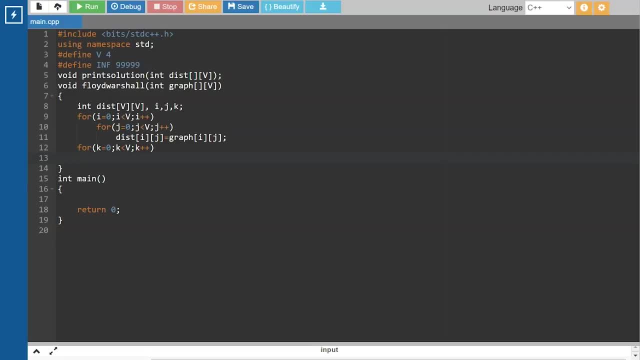 Now we will pick all vertices as source, one by one. i is equal to 0,i less than V, i plus plus. Now we will pick all vertices as destination for the above picked source. So for: j is equal to 0,j less than capital, Vj plus plus. 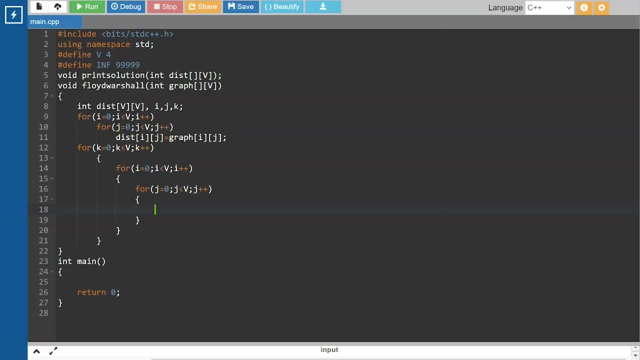 Now, if vertex k is on the shortest path from i to j, then we will update the value of distance i comma j. So if distance at i comma j is greater than Distance at i comma k plus distance at k comma j, And distance at k comma j is not equal to i and f. 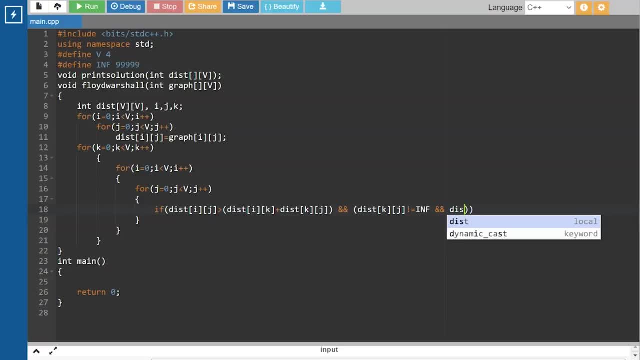 And distance at i comma j is equal to i and f. i comma k is also not equal to i and f, Then distance at i comma j will be equal to distance at i comma k plus distance at k comma j. And distance at i comma j is equal to distance at k comma j plus distance at k comma j. 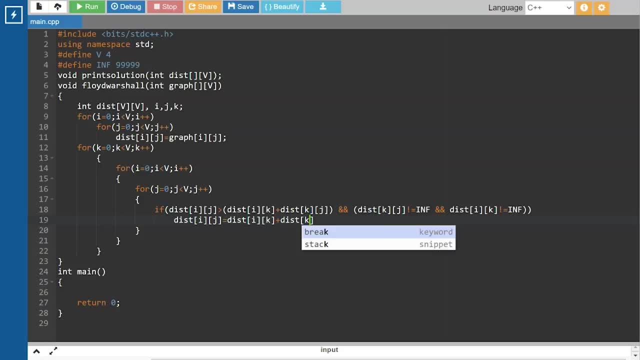 distance at kj. now we will call the print solution function for test. now let's write the utility function to print solution. so void print solution and test. we will start with cout. the following matrix will show the shortest distance between every pairs of vertices for loop: and I is equal to 0, I less than. 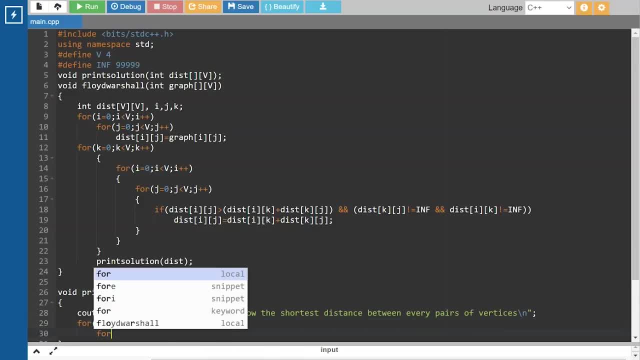 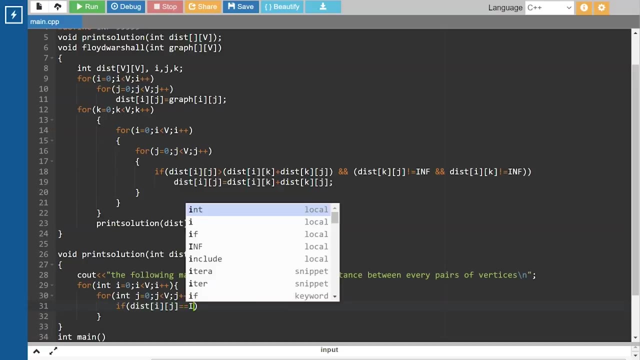 capital V I plus plus for loop, and J is equal to 0 J less than V J plus plus. if distance at I comma J is equal to INF, then we will see out INF, else we will see out the distance at I comma J. now we will see.